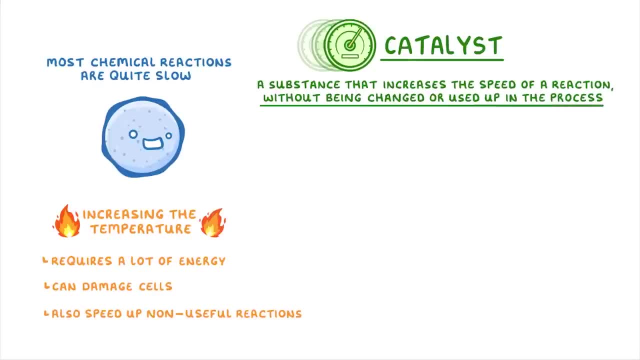 used up Now. the word catalyst is a general term that you might see in chemistry as well, But an enzyme is a particular type of catalyst that's made by living organisms, and so we sometimes call them biological catalysts. Enzymes themselves are basically just large. 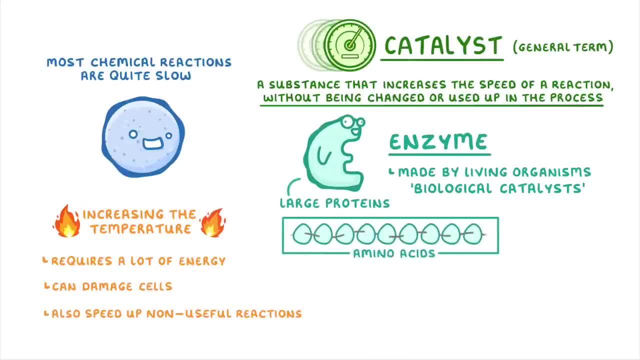 proteins. So, like all proteins, they're made up of long chains of amino acids And, depending on the specific sequence of amino acids in the chain, they can fold up to form different shapes, And each of these shapes would be a unique enzyme that catalyzes a 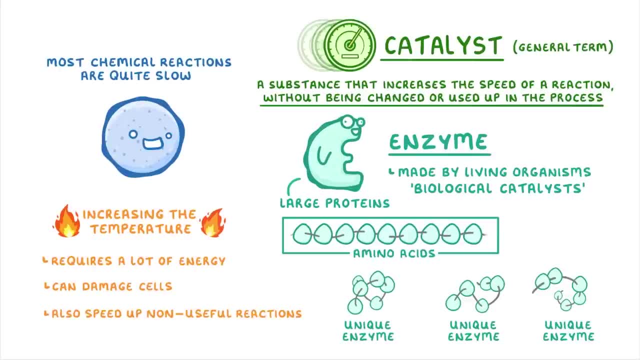 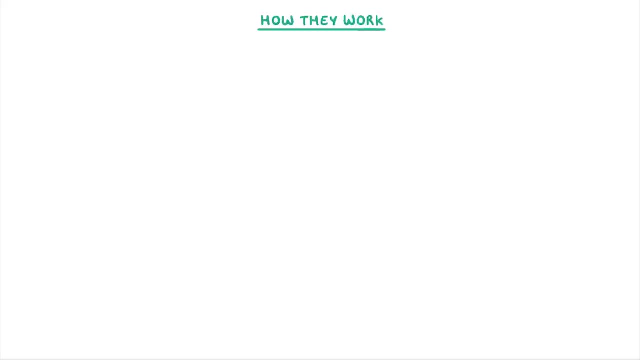 particular chemical reaction. So now that we know what enzymes are, we need to look at how they work. If you think about chemical reactions, they often involve taking a chemical reaction and then taking it to a different enzyme, And that's what a catalyst is. So now that we know what enzymes are, we 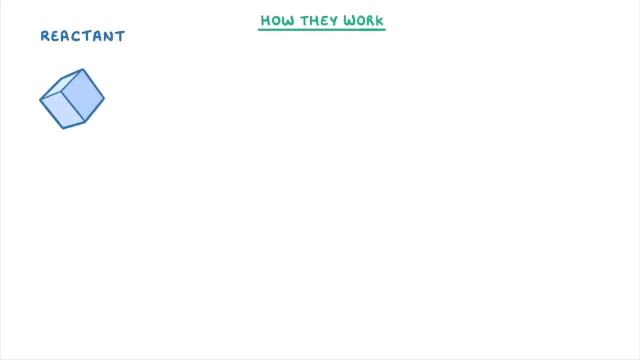 need to look at how they work. If you think about chemical reactions, they often involve taking a reactant, which, in biology, we can call a substrate, and breaking it apart into smaller pieces, which we can call products, And the reverse is also very common with 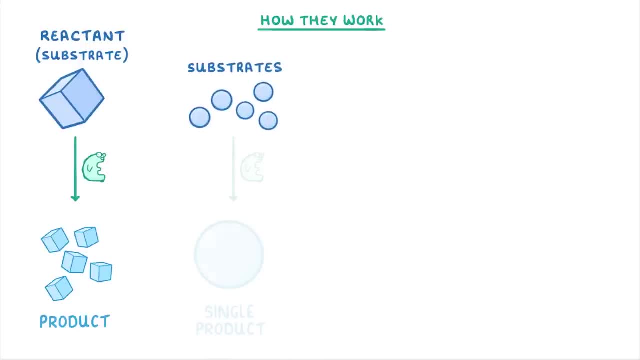 chemical reactions joining together multiple substrates into a single product. The important thing to remember is that all enzymes do in these cases is speed up the process, And to do this they have a special region called an active site, which is a part of the enzyme. 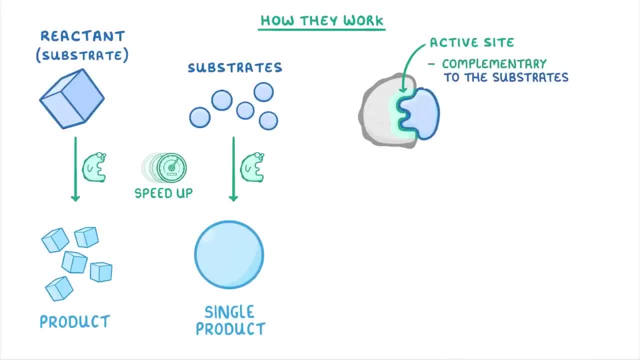 unique shape that's complementary to the substrates of the reaction, And this point is really important. If the substrate doesn't fit the active site of the enzyme, then the reaction won't be catalyzed And this allows the enzymes to be really specific. 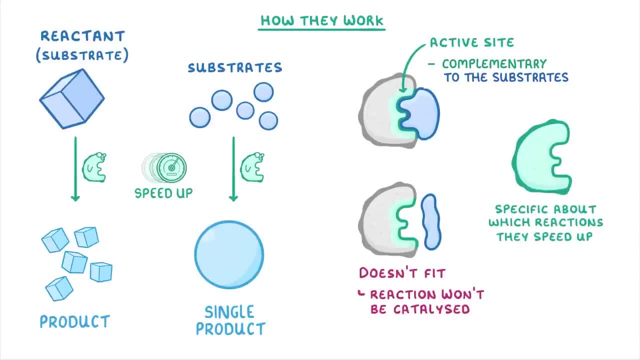 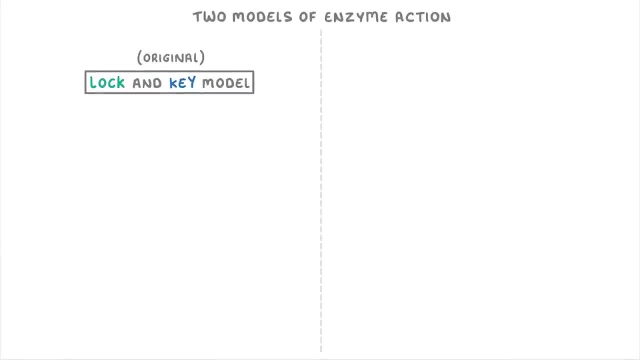 about which reactions they speed up. The very last thing we need to cover are the two models of enzyme action, So the original lock-and-key model and the more realistic induced-fits model. At first, scientists thought that the substrate had to fit perfectly into the active site, just like how a key fits. 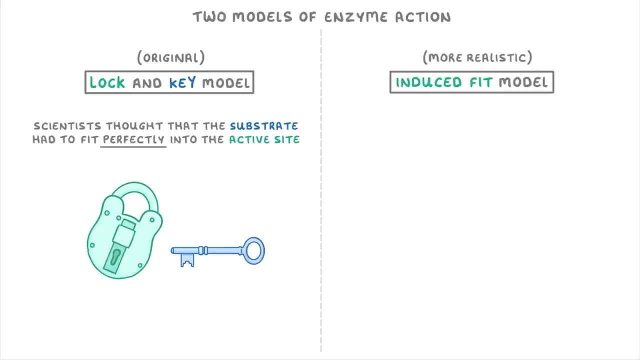 perfectly into a lock, Hence the name lock-and-key model. However, we now know that the enzyme actually changes shape slightly as it binds to the substrate so that they can fit together more perfectly In exams. you want to describe this by saying that the active site is called.